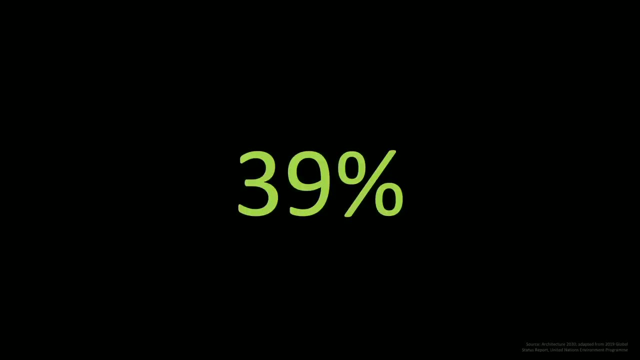 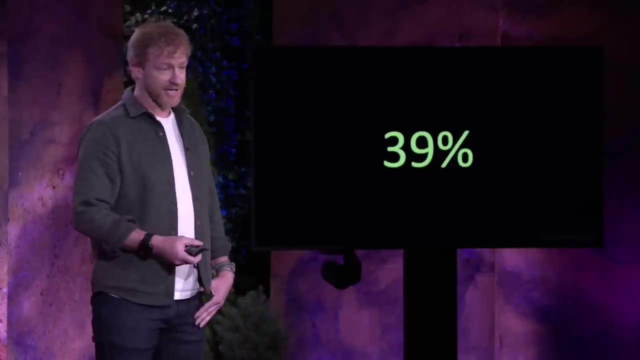 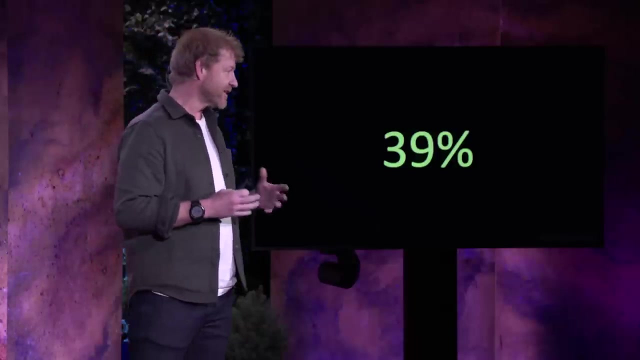 goes into the built environment. The other challenge with buildings is they represent about 39% of our greenhouse gas emissions, or, in North America, almost half of our greenhouse gas emissions. For reference, because it's not talked about enough- all of cars, planes, automobiles, the entire transportation sector combined. 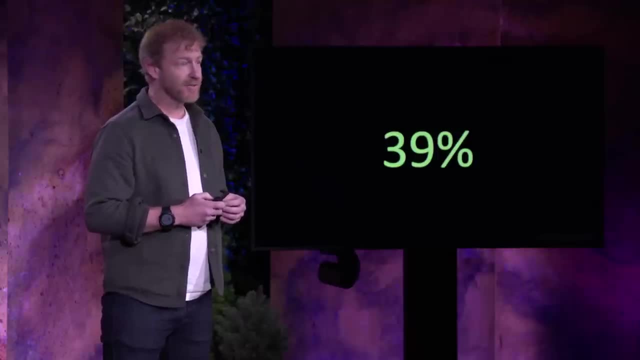 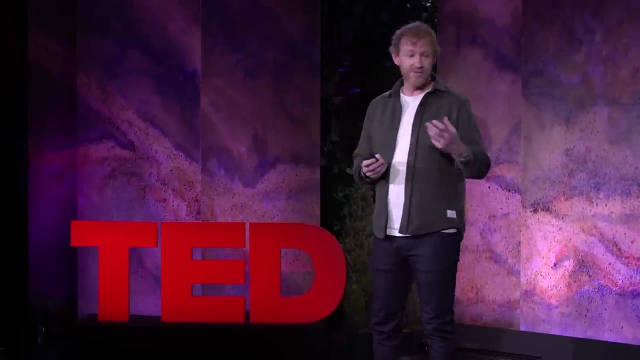 represent only about 23%. So buildings are a huge part of the problem and not discussed enough. The reason for that are both the heating and cooling of buildings, of course, but also the materials that go into buildings. So, when it comes to materials, 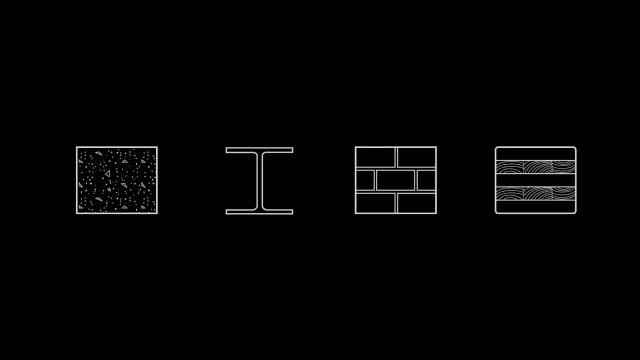 the building structures. what holds the buildings up really are composed of four major materials in every city on the planet: Concrete, steel, masonry and wood. And of those four materials, three of them have very, very high carbon footprints. 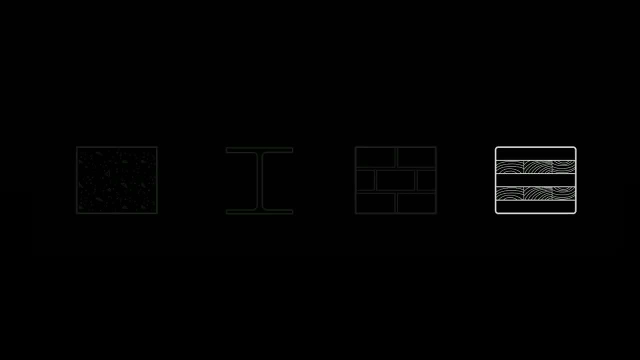 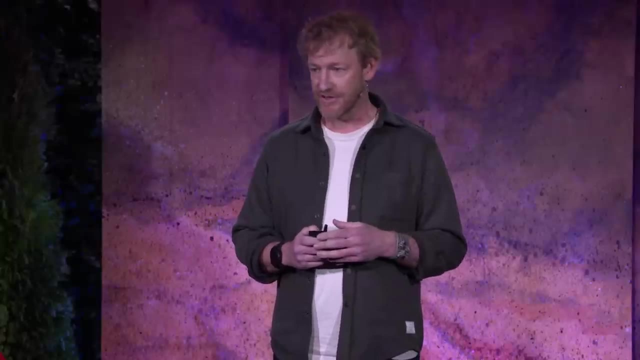 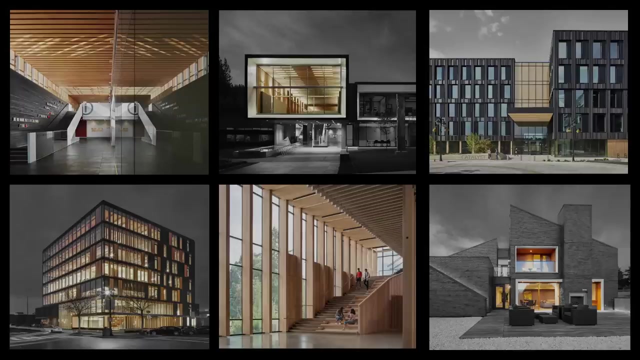 in particular, concrete and steel. Now, wood is the only material on that list that's also a renewable resource and sequesters carbon, So it's the only pathway as a material that actually can get us to carbon-neutral buildings, And it's the pathway we choose in our practice to build all buildings. 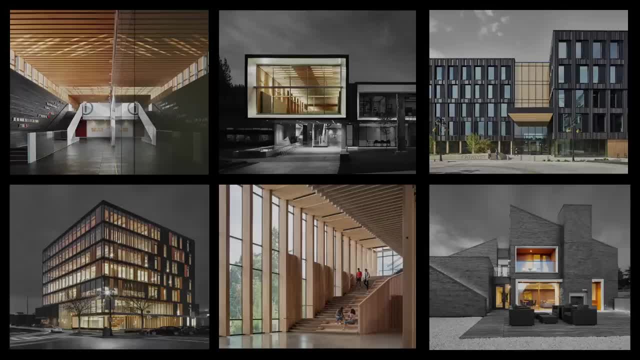 So our practice has been a timber-only practice since our inception And as part of our advocacy for the use of wood in buildings, about 15 years ago I wrote a book called The Case for Tall Wood Buildings, And that book taught the lesson of why we should do this. 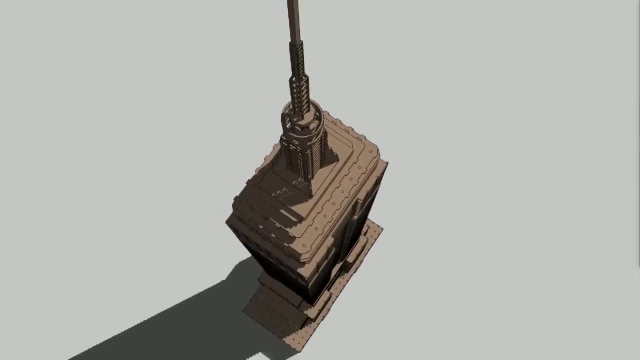 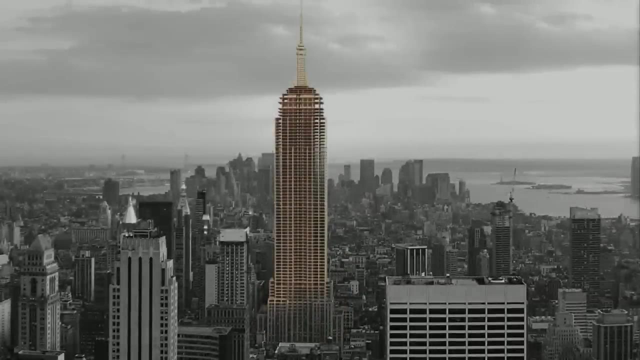 and how we should do this, And in the beginning it was a very unlikely concept that people had a hard time believing. And, yes, we figured out that we could have built the Empire State Building entirely out of wood. That early idea now is a mainstream concept around the world. 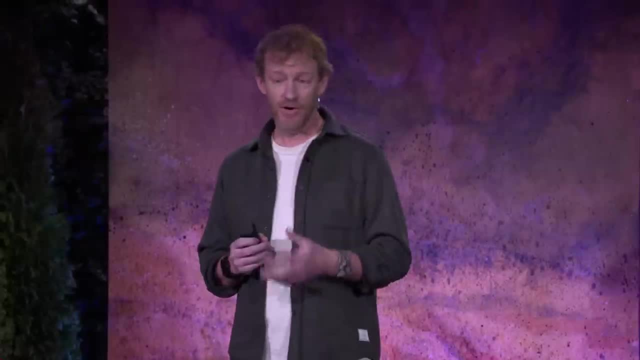 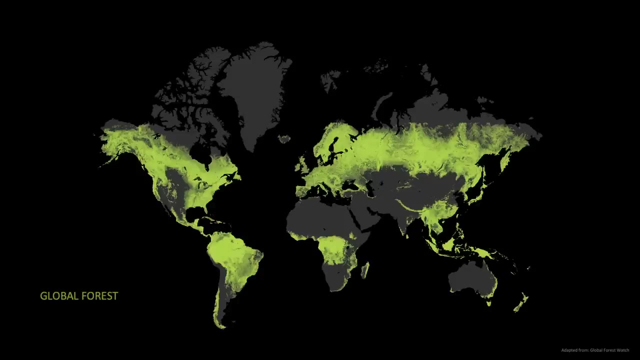 in sustainable building practices, and there are hundreds of tall wood buildings that have either been built or are currently under design and construction, and thousands more to come. But wood as a sustainable idea is not sustainable unless it actually comes from sustainable forest practices. 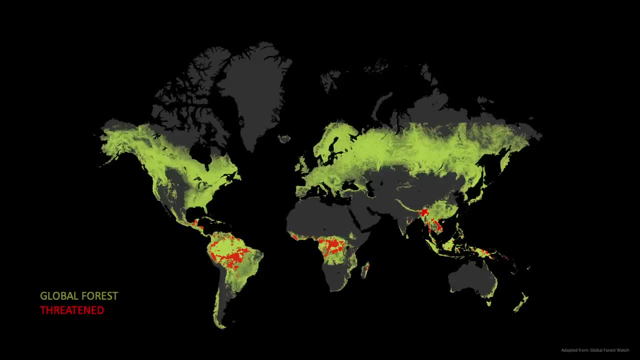 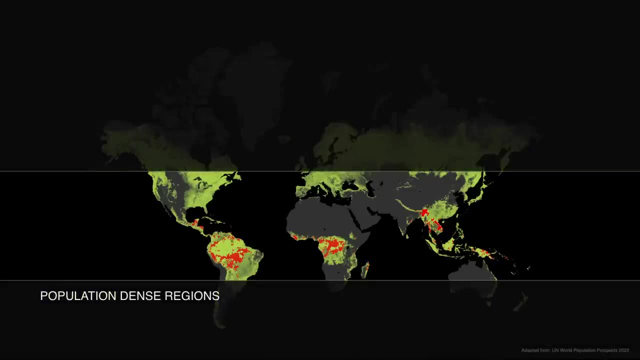 And much of the planet has forests that we actually need to keep standing as part of our climate solution And, in fact, lots of the world have forests that are under deep threat, If we think about where population in the world mostly resides and where it's growing the quickest. 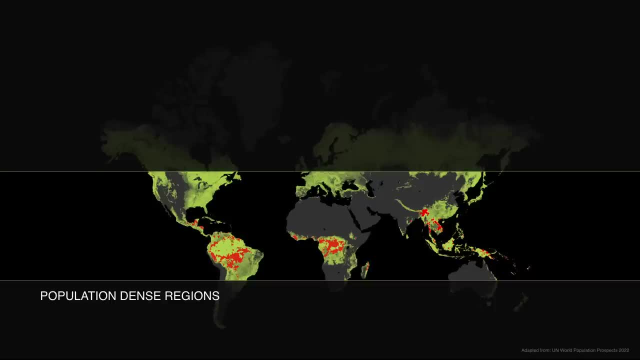 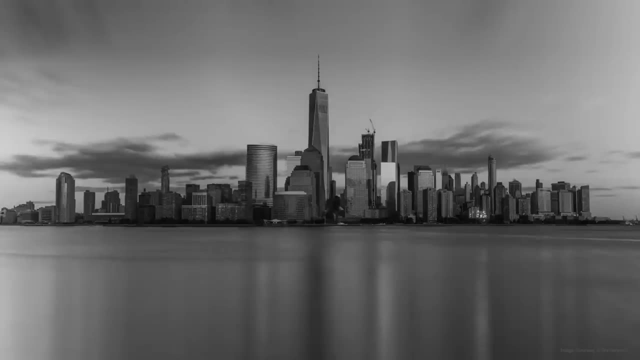 in fact, most of those areas either don't have forests or also are where these forests are threatened, And so wood is good. As good a solution as it is, and a solution that I still very much believe in, is not a global solution. 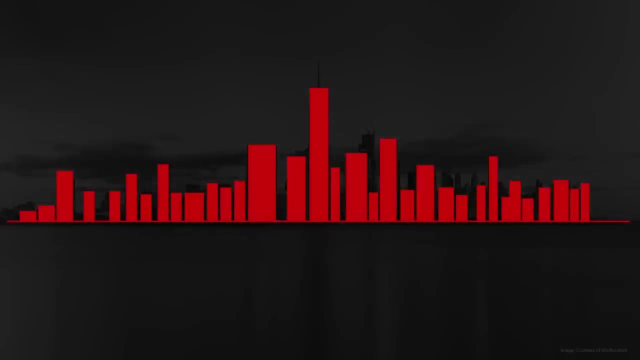 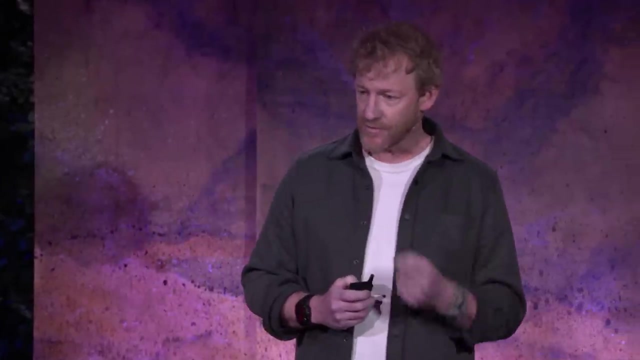 Most of our cities are still built on those first three materials- steel, concrete and masonry- and they have a high carbon footprint. We're working hard and people are working hard to make concrete and steel better, but unfortunately tweaking those existing materials. 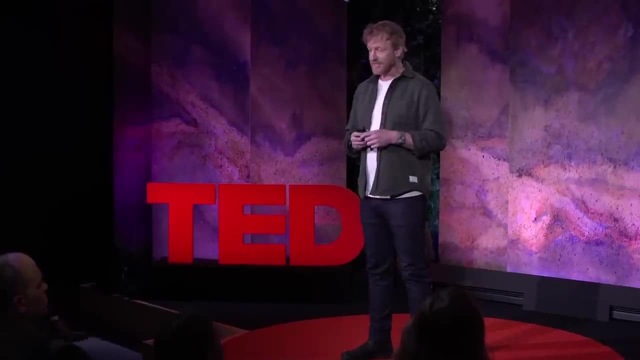 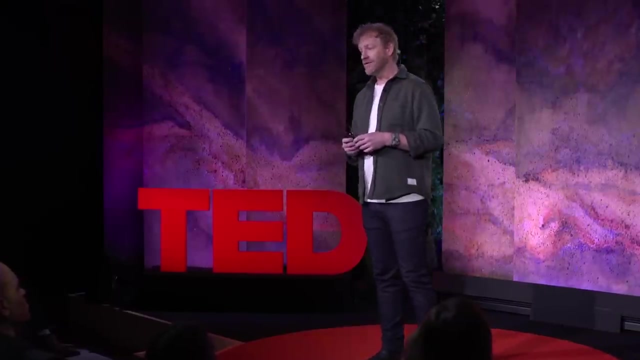 is making them only modestly better. In the case of concrete, it's estimated they can reduce the carbon footprint of concrete at best between 10 and 35 percent, And that's a long way to go from where we need to be either at carbon neutrality in our cities. 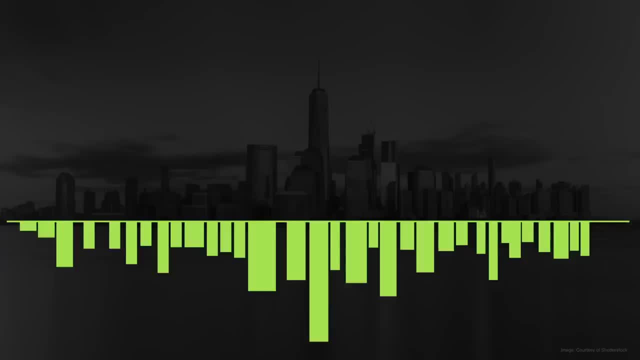 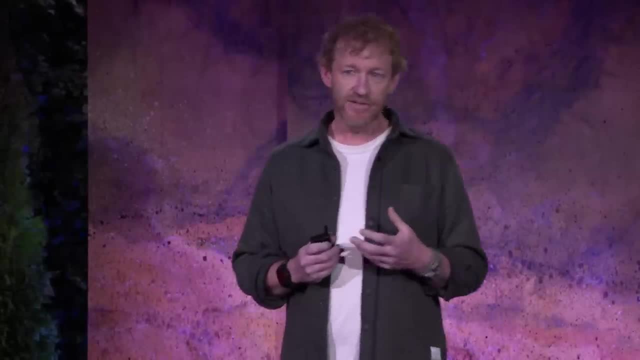 or, better yet, in carbon sequestering, carbon-negative buildings. So how do we get there? After building about a million and a half square feet of mass timber? I still believe in that material, but I keep asking myself this question: What is the alternative to the big four? 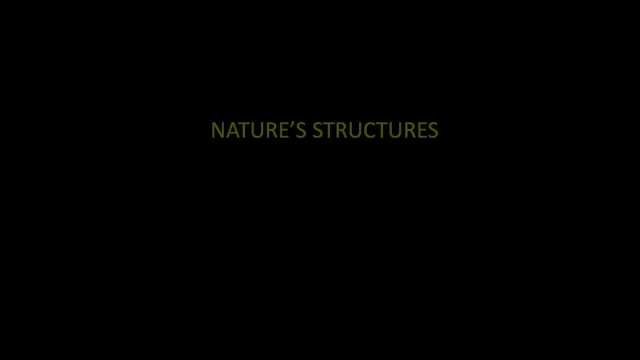 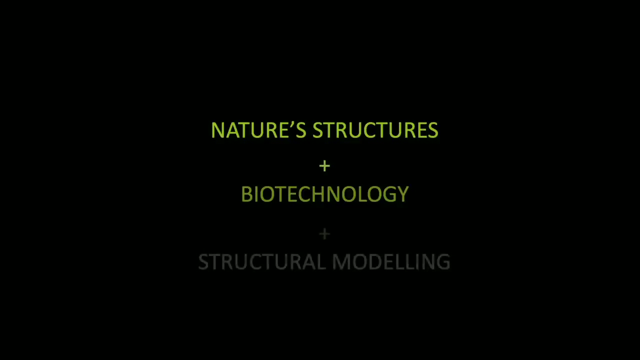 And the answer in my mind, without question, is studying and understanding what's happening in nature and nature's structures, combining that with modern biotechnology and combining that with all of the computer modeling that allows us to make incredibly efficient structures going forward. 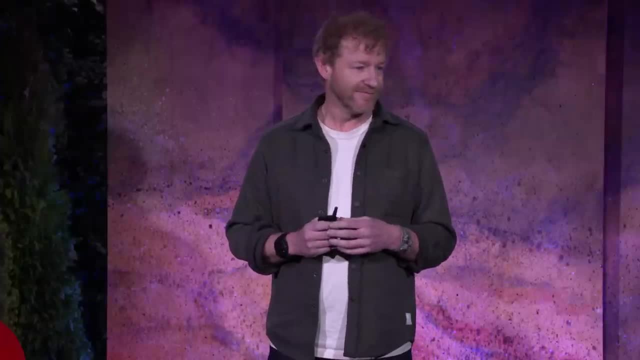 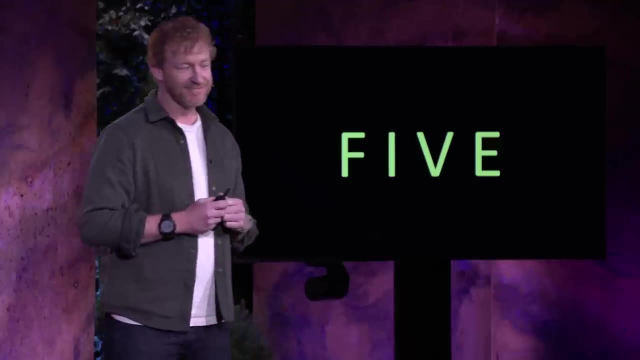 All those things together are creating what we call five. Five is a fifth way, a new structural material that will replace in my mind, over time, the big four. It's an all-organic material made from forests and crops that can be grown all over the world. 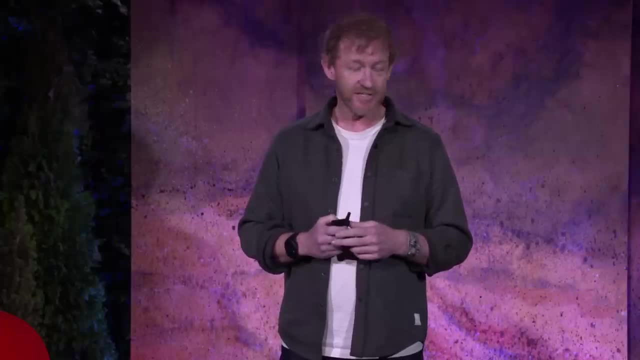 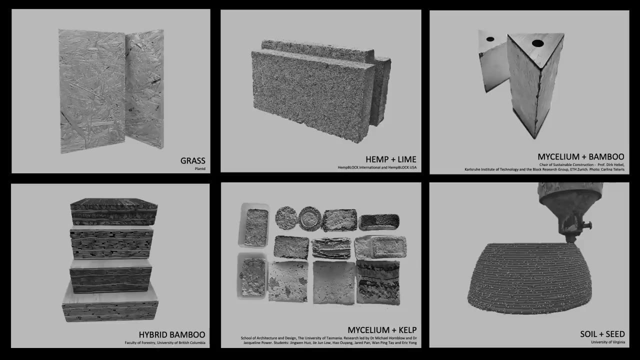 It's strong and safe, and it eventually will be cost-effective and competitive against any other material. Now, this isn't a new idea. Products made from natural materials, thankfully, are growing up everywhere. There's a huge industry of biomaterials in academia as well as in private business. 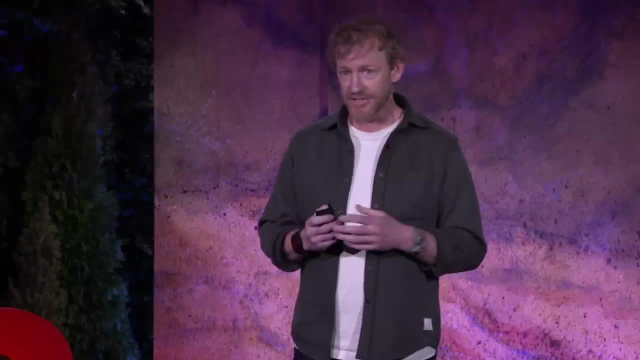 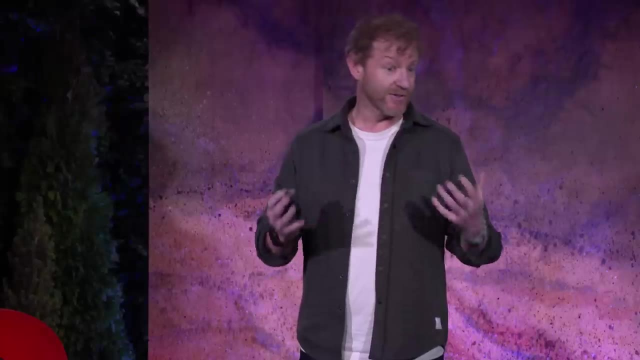 and we're seeing new products come online every day. This community is strong and hopefully getting stronger, and our contribution to it is really focused on this idea of the biggest material use, which, again, is the building structure. So how does it work? 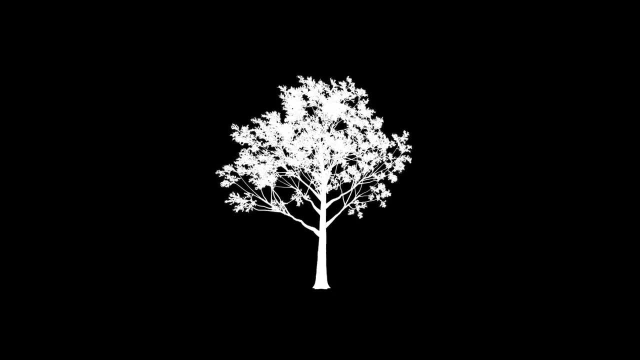 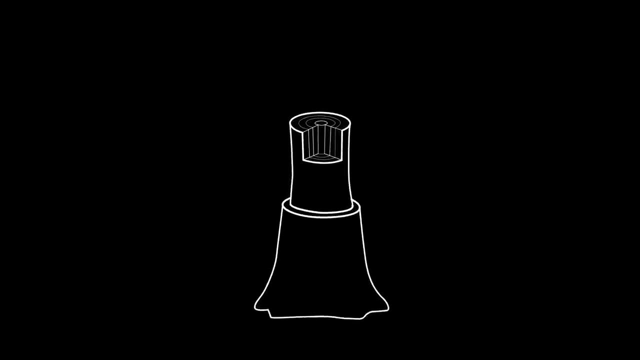 So the idea is based on the same concept of how a tree works, or any other vascular plant As we zoom in. a tree is sort of made of lignified tissues that go from the bottom of the tree to the top, as are plants. 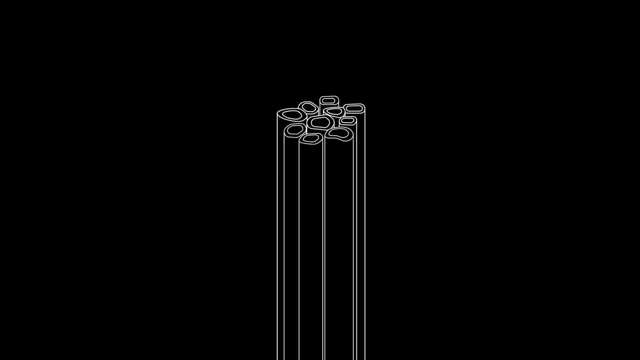 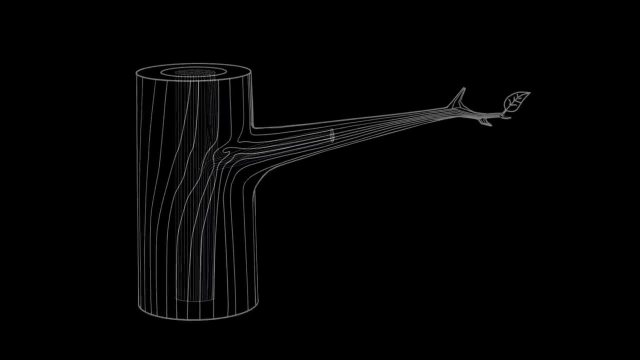 And those lignified tissues have within them, in the cell structure, cellulose fibers and lignin that together make the plant strong in order to grow and thrive. And those two materials, the fiber in the plant, as well as the lignin, as well as other binders. 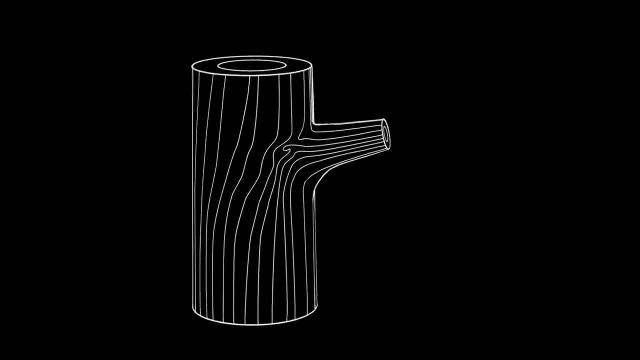 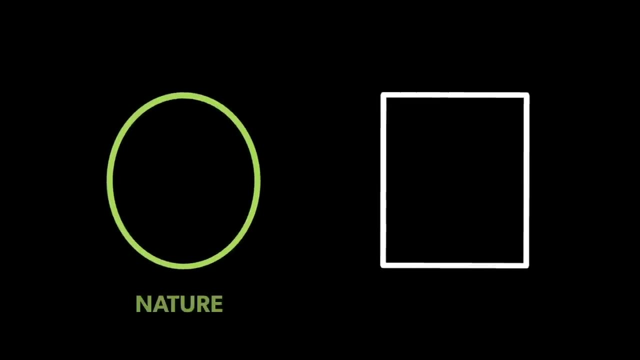 make up the ingredients of what we call five. Studying the fibers and how they work in plants is another part of how we're trying to make this structure. And if we all imagine cutting through a branch, as the image just showed, we know that nature finds very efficient ways to create structures. 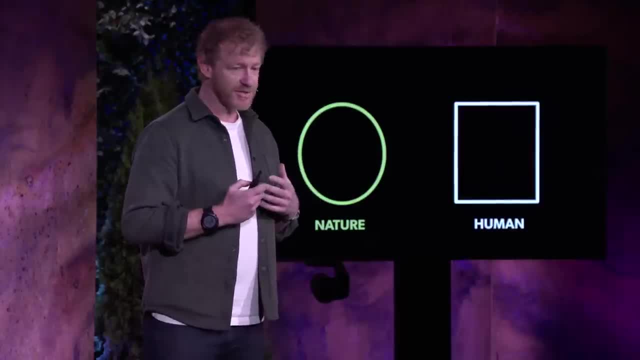 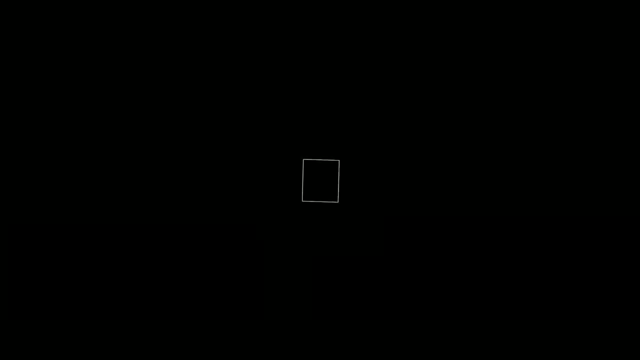 and they're often round like a branch, But as humans we tend to make boxy structures, And the reason we do that is concrete. steel and these materials in wood are more efficient when we form them as a box or when we cut them as a box. 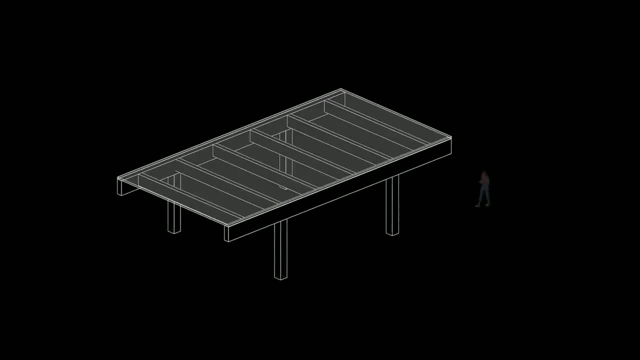 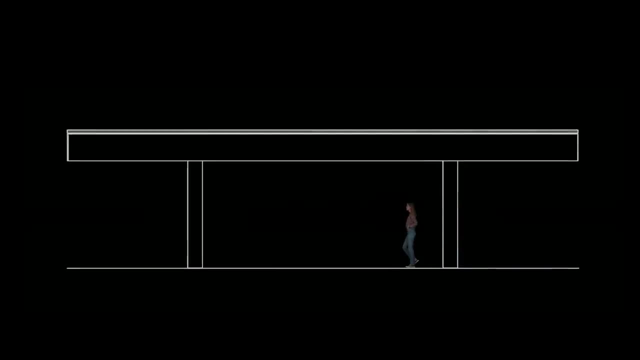 It's more affordable and that's why we see it. So a typical structure has columns and beams and a slab that make it up, And they're very boxy forms. as you can see in the image Now, different structures behave very differently all the time. 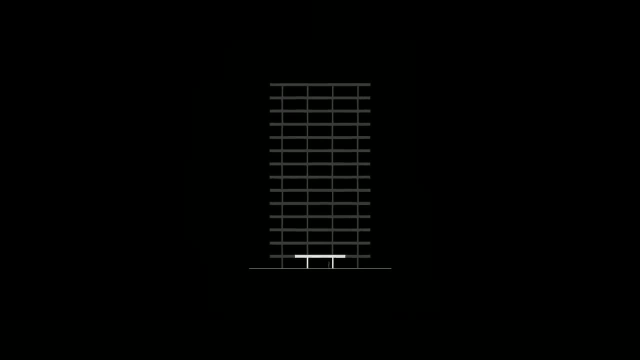 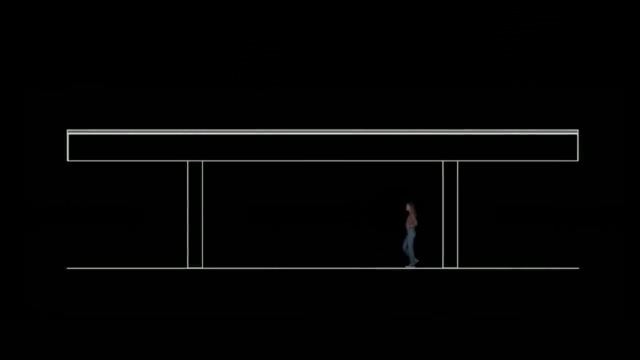 This particular structure is an example from a tall building, but if we were talking about a house, it would be a different structure. or if we were talking about a hockey rink, it would be another structure. So, just in this example, how do the forces work? 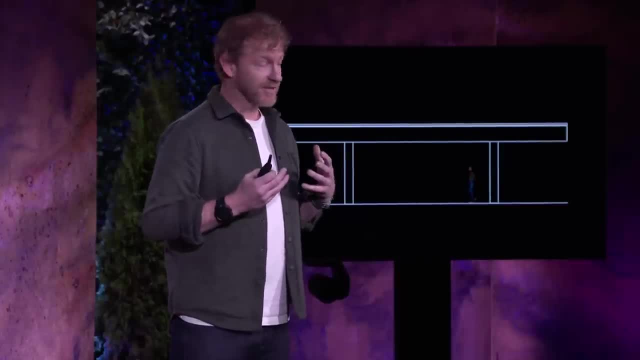 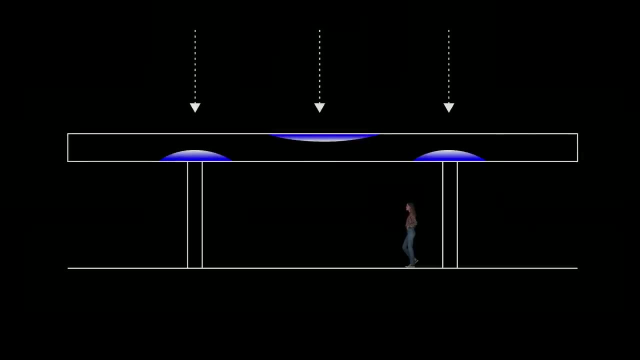 Well, you have the force of the weight of people and you have the force of the weight of the building above. You have wind blowing on the sides or an earthquake impacting it. The forces as they press down on this particular example in blue are forces of compression. 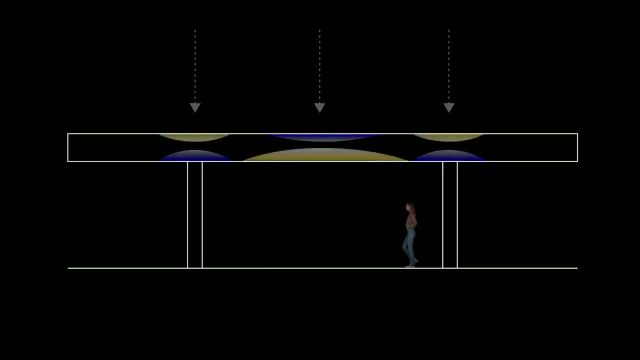 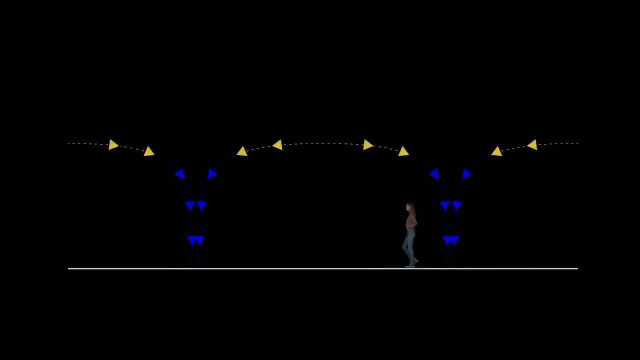 That's the squeezing forces pushing down, And the forces here in yellow are the tension forces, the pulling apart on that structure. When we put those together, we see how the forces move to the ground through this simple frame and it's sort of a flowing diagram. 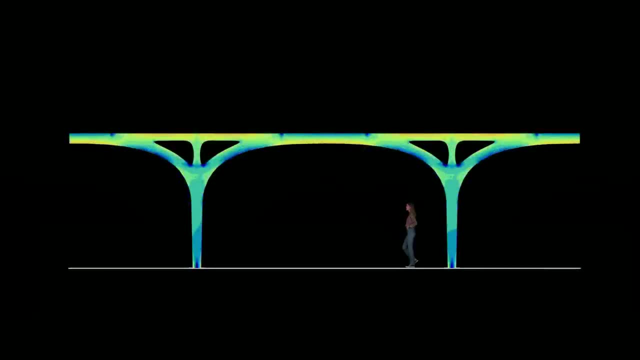 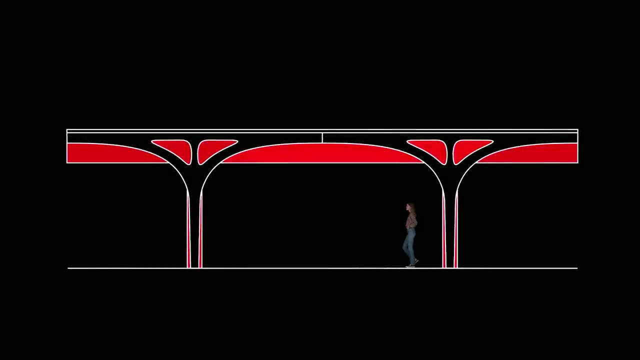 In fact, when we use what's called a structural stress plot, you can see that the form is very natural in its character. But, as I said, we build things out of boxes And when we overlap, in our example, a boxy structure of wood, for example. 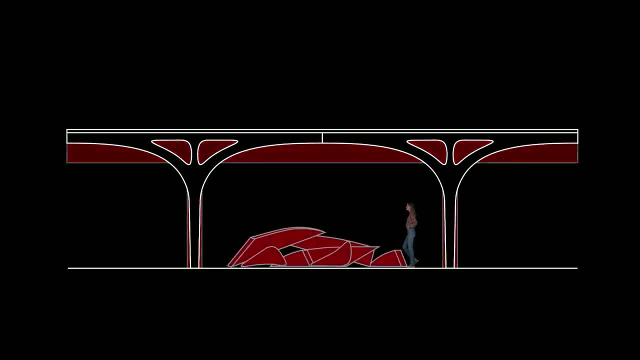 we see these areas in red which really are unnecessary. They're wasted material in the current way we build. In this example. working with our engineers, we actually calculated that this particular example would result in about 27 percent material waste. Now, all buildings are different. 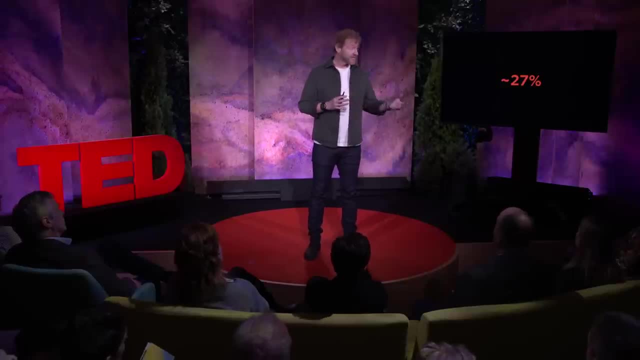 and it's very hard to make a sort of overall calculation. some buildings are more efficient, some less efficient, But if we multiply this by the amount of building that needs to be built over the next 40 years for humanity, it's an incredible amount of human waste. 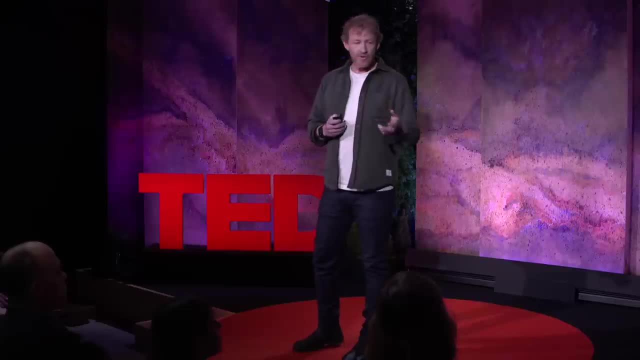 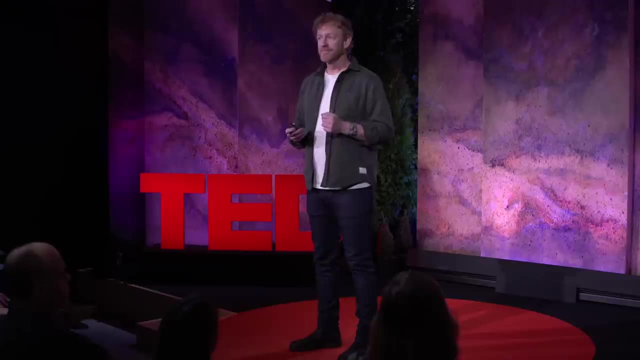 and poor use of our resources. So our goal with five is: how do we use as little resources as possible? And when you use little resources in a building, you lighten the building up, And a lighter building actually means that it weighs less on the ground. 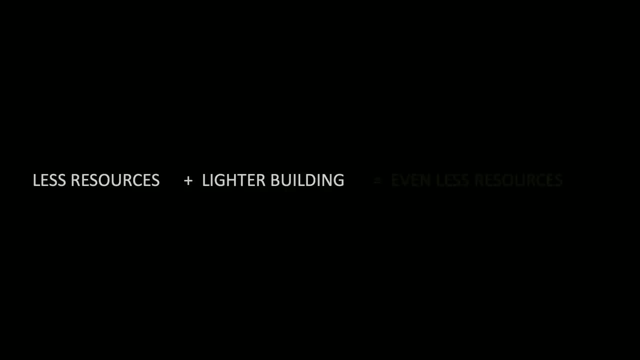 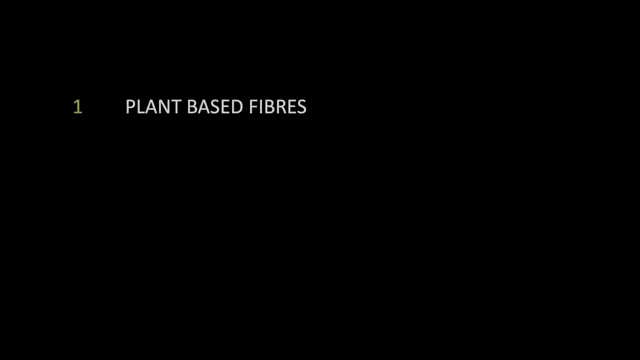 and our foundations below the ground can be lighter as well. So less resources equals lighter buildings equals even less resources. Taking this idea of how five can use less, we took four existing known solutions and put them together. The first is we take those plant fibers I described. 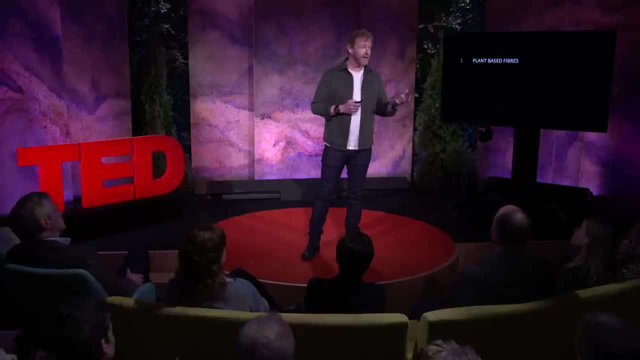 and that can come from trees, that can come from plants, grass, bamboo, It can come from waste wood products. It can come from clearing the understory of a forest to make it less likely for forest fire. in places like California, We take those fibers. 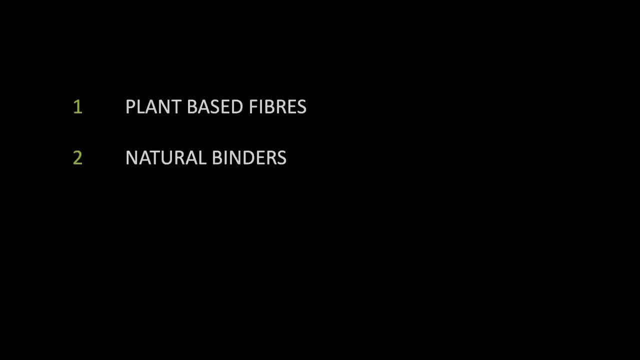 and combine them with other organic binders and lignin in order to sort of create a solid product. And then we take these computer models that allow us to really design efficiency into the way we build, so we can boil out all that waste. And then finally, we're going to use custom robotics. 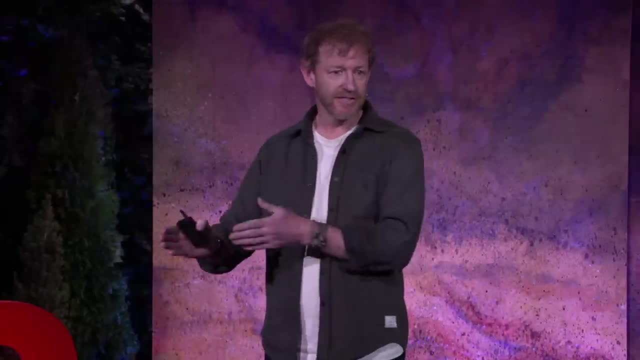 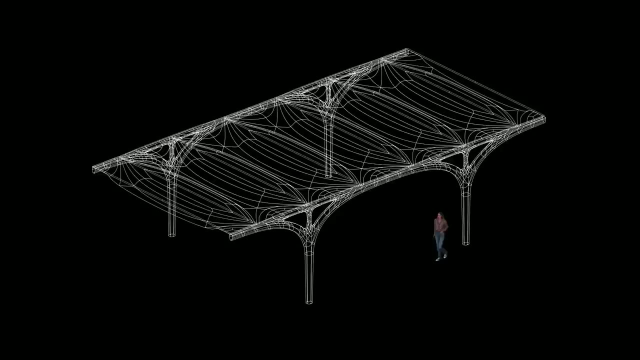 that means that every part of a building, rather than being cookie-cutter and the same and wasteful, can be just as much material as needed, and no more, in order to make the building safe. Together, that makes something that looks like this: 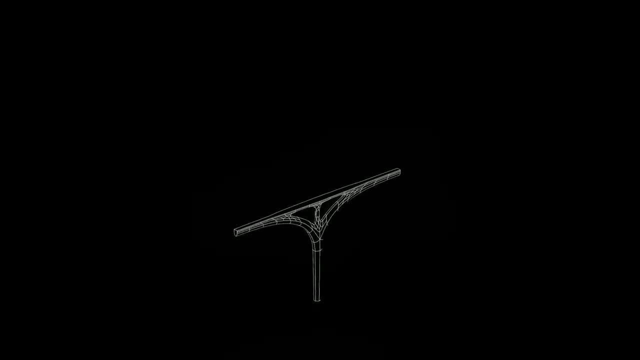 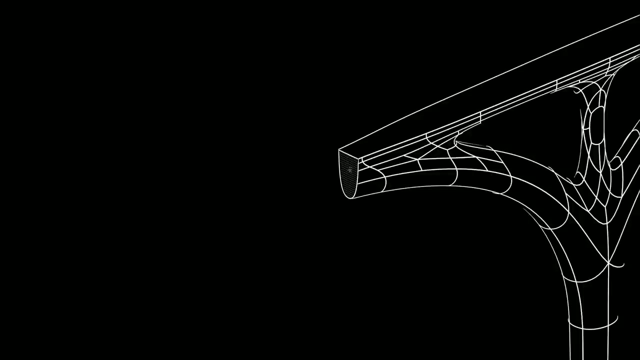 And again, this is an example. The flat top is flat because we walk on floors, but underneath the building looks more organic in its shape And, as you can see, these beams and columns feel a little bit more like branches and more like what we see in nature. 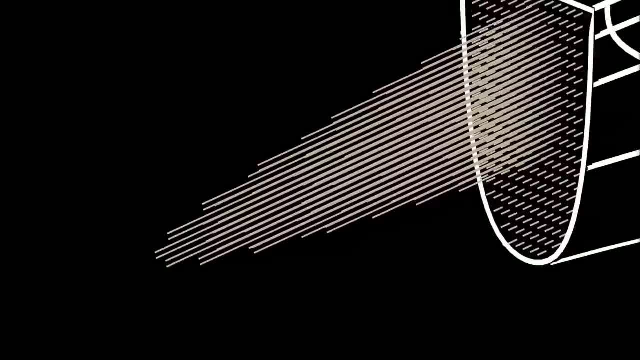 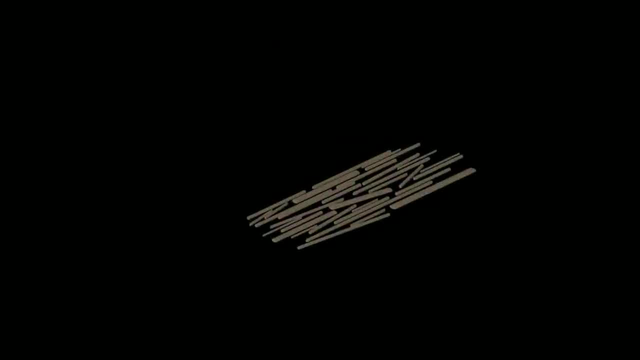 As we zoom in even further, we start to see how it's actually composed. And you may think in your mind: is this fiberboard? is this particleboard? things you've seen before? Well, actually, what we're talking about is a very microscopic layering of these plant fibers. 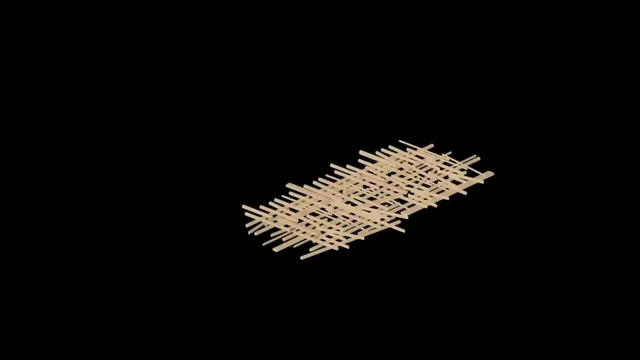 They're just a millimeter long. By laying them together and cross-laminating them across each other, we can customize the way, based again on the structural model, exactly how the composition of each piece of the material works in order to make it as efficient as possible. 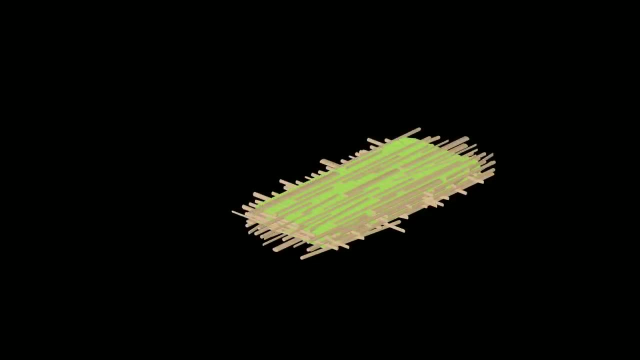 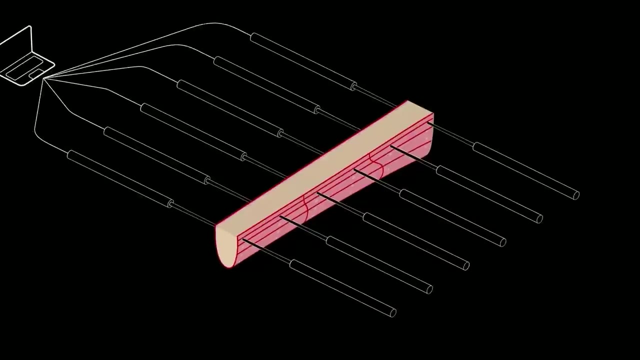 We combine it with these organic polymers and lignin and ultimately make this material as strong, dense and behaves much like a tree would. Now we do that in another unique way, in the way the forming works, Because no pieces of a structure have to be the same. 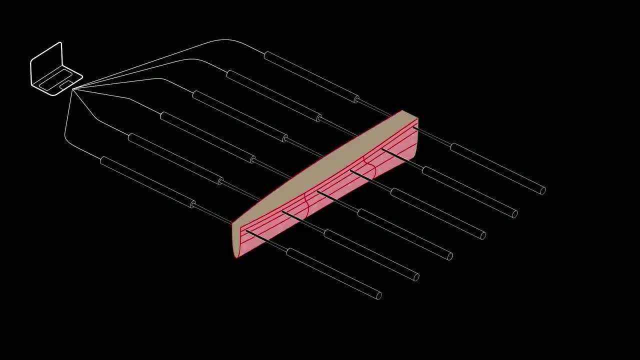 and we want to reduce waste. we use robotic forms and fabric forms. The red is fabric that moves in and out and allows each piece of the building to be completely uniquely customizable, And again, we're using it to reduce the waste of a structure. 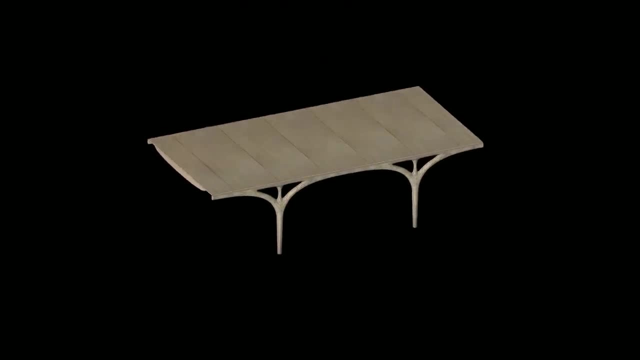 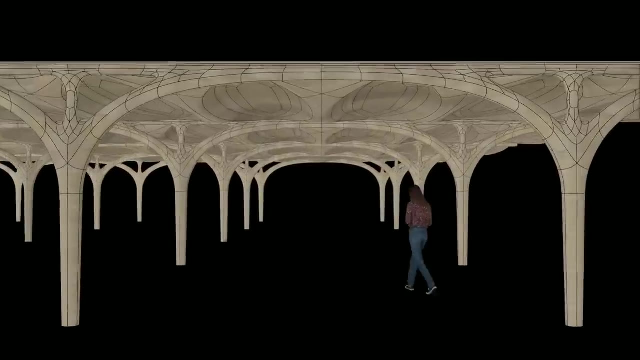 Now, when we put that all together, it looks like something completely different, something that none of us have seen before. It's not like steel, it's not like concrete and it's not like wood. Instead, in this example, what you see is an entirely plant-based structure. 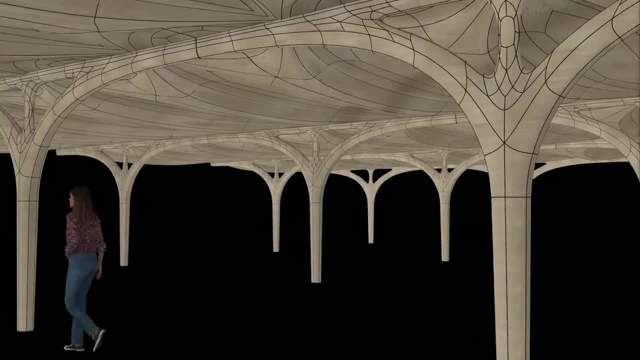 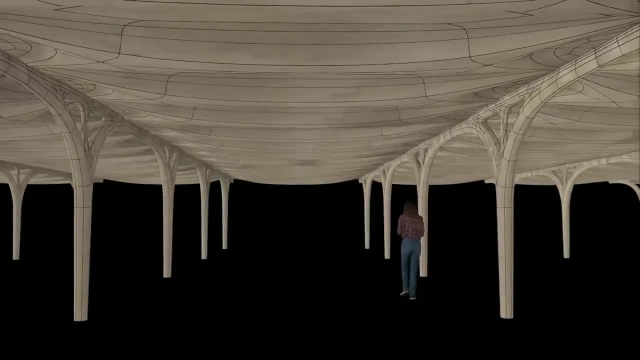 It's healthy and beautiful to be around. Its shapes are not there as decoration. they're there as just structural essentials, and yet they're beautiful. It's safe to be within. It sequesters carbon, so it's part of our solution for climate change. 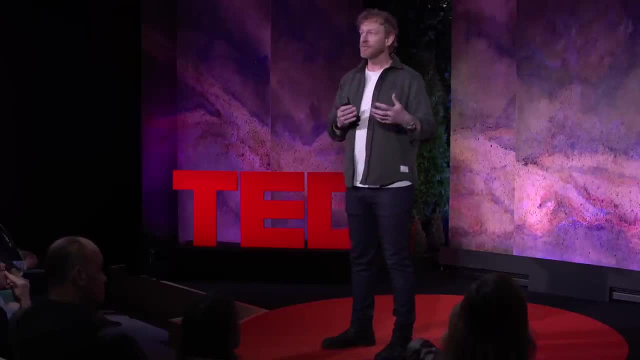 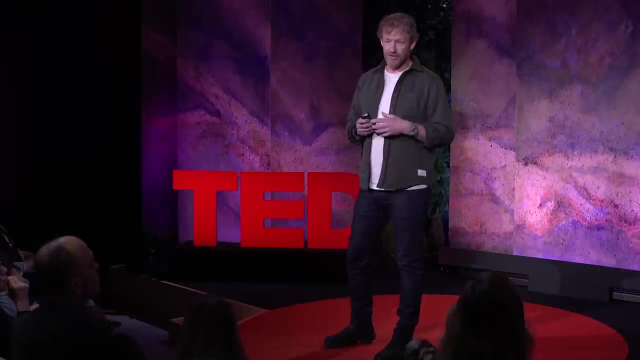 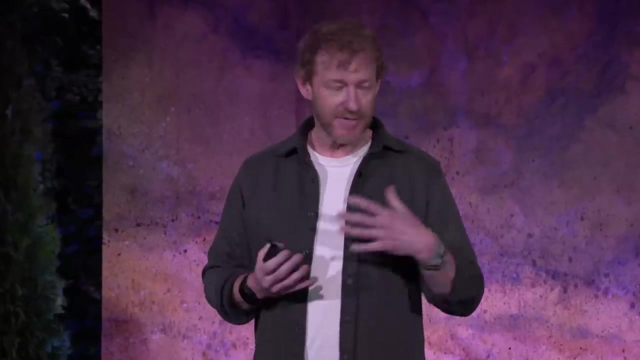 I believe we cannot continue to work with broken systems and try to make them better. We have to imagine something next. We also can't wait for the world's resources to run out before we imagine a future that's different. We're no longer part of an industrial revolution of materials. 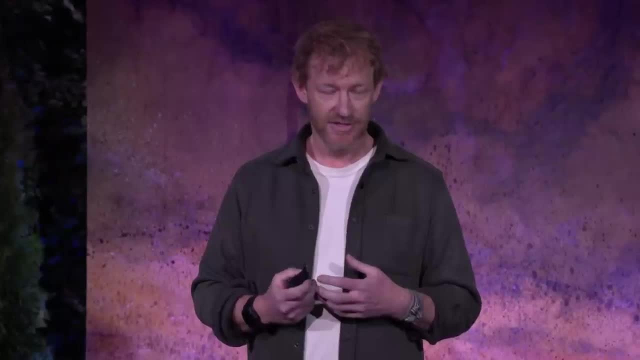 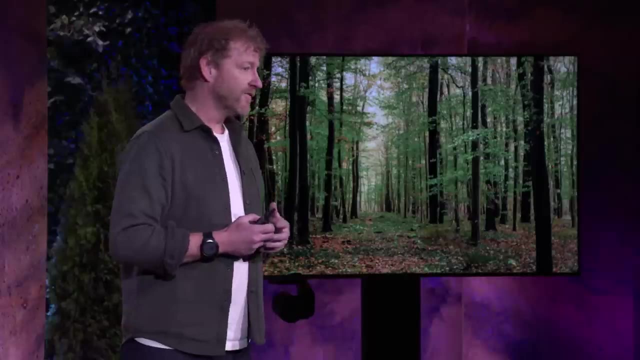 we are at the beginning of Mother Nature's revolution of materials And, as a result, we can make much more beautiful environments for everyone. As I walk around the forest of my home and I look up into the trees and imagine what the buildings of the future are.